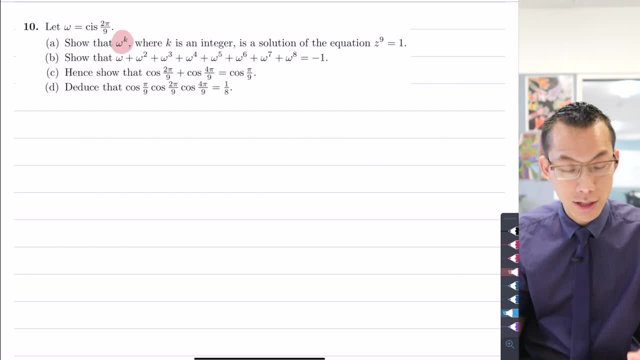 that. And then, secondly, what does it mean for some complex number like omega to the power of k? what does it mean for it to be a solution of the equation z to the nine e? How do we go about showing that? So let's begin with part a. I'm going to write this out in long. 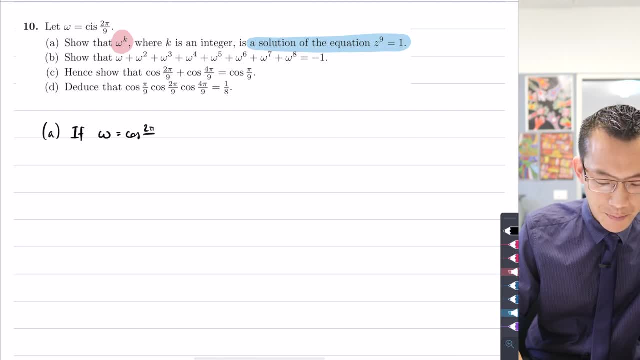 form. omega equals cos two pi m nine plus i sine two pi m nine. And then what I want to think about is: well, what piece of knowledge or what skill do I have access to that enables me to raise a complex number to an integer power? And hopefully your brain is going there. It's going to be. 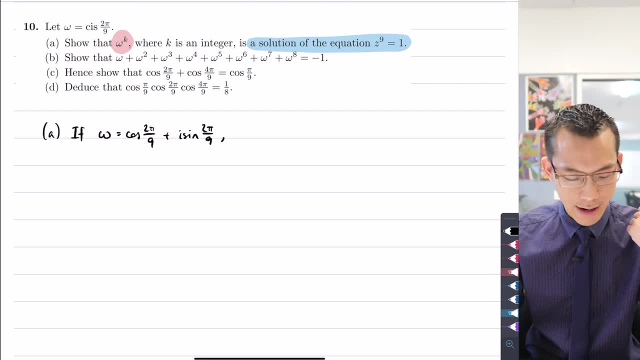 de Maverick's theorem right. So I'm going to say: if this is omega, then omega to the power of k is going to be equal to. you recall that this raising to a power multiplies these two arguments here by whatever power we raised to. So I'm going to write that as: 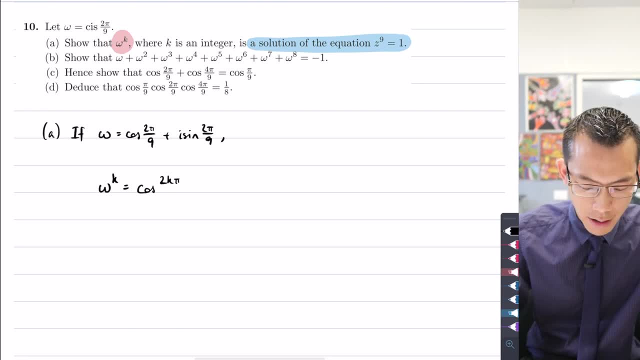 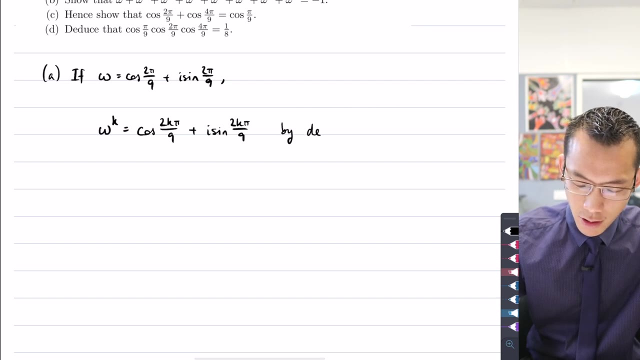 cos two k pi on nine. That's probably the most natural way to write it. Plus i sine two k pi on nine. And this doesn't come out of thin air, It comes by de Maverick's theorem. So I should quote that right. So I'm going to say by de Maverick's theorem. 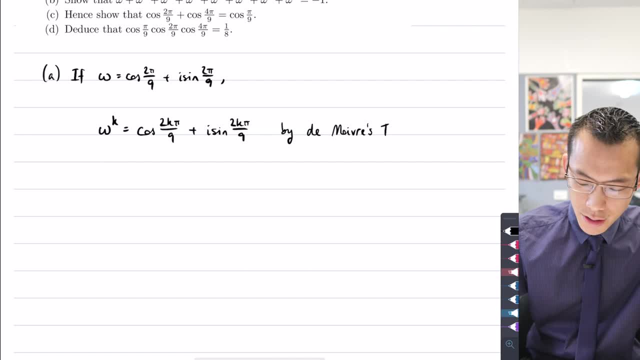 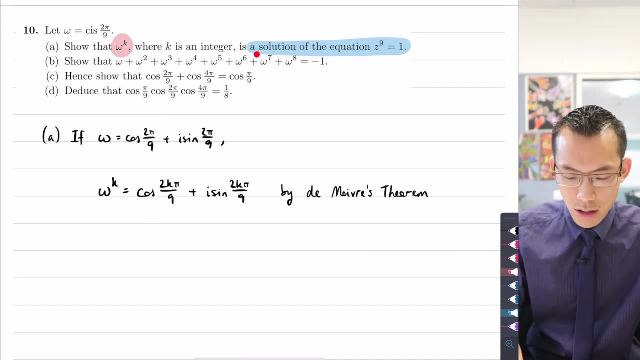 So this is settled for me, what omega to the power of k is. And then I want to say: well, how do I show that this is a solution of the equation? z to the nine equals one. Well, I can actually go a little bit further here, because I actually know a lot about what happens when you have some 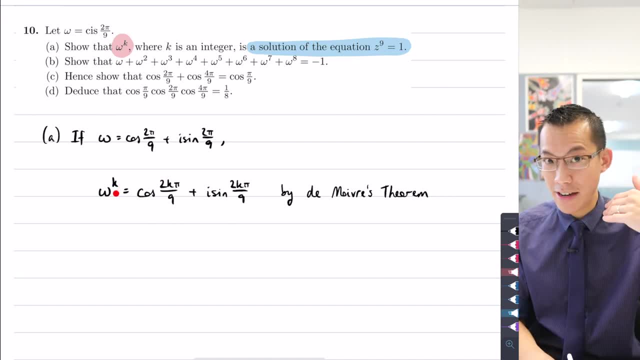 multiple here and raise it to the power nine. I'm not just raising it to the power of k, which is the first use of de Maverick's theorem. I'm going to raise that to the power of nine, because to be a solution of an equation means substituting in that particular value will make the equation. 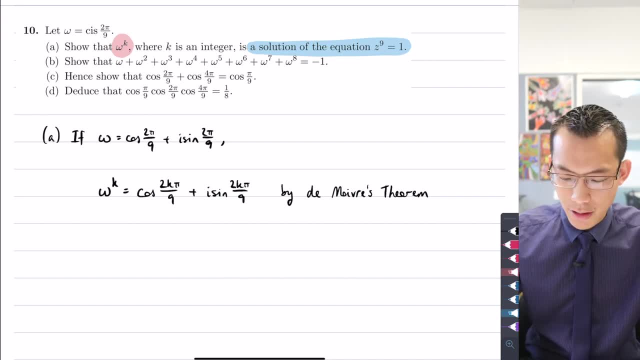 true, It will satisfy the equation. That's what we mean when we say something like: oh, what are the solutions of an equation like this? The solutions are: x equals negative two and x equals negative three, a factor you would arrive at by factorizing, That's an x plus two and x plus three, So it can. 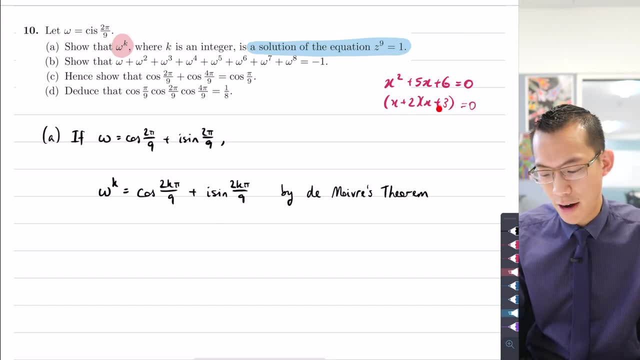 be clearly shown by putting in negative two. It doesn't matter what happens to this second factor. zero times anything does indeed equal zero. So what we're trying to show is that if I put this into here, raise it to the power of nine, I should get one. Well, that means I've got to use a second. 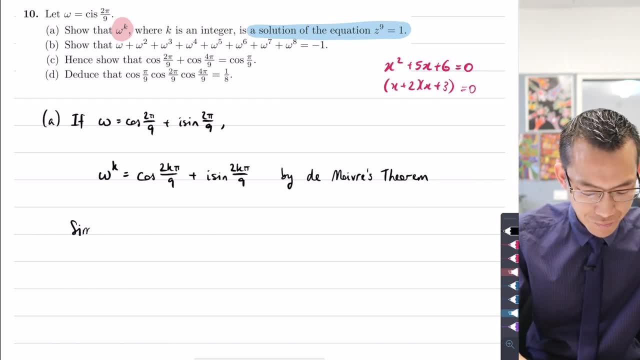 application of de Maverick's theorem. So what I'll say is: similarly- and now I'm going to- that's very messy- raise this thing here to the power of nine, I will get omega to the power of k, to the power of nine equals. And now, just like before, I am going to multiply these things by: 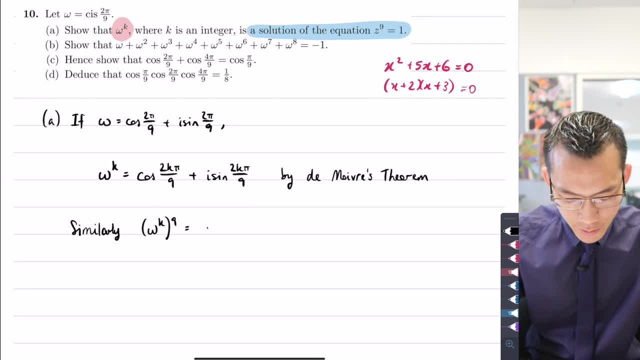 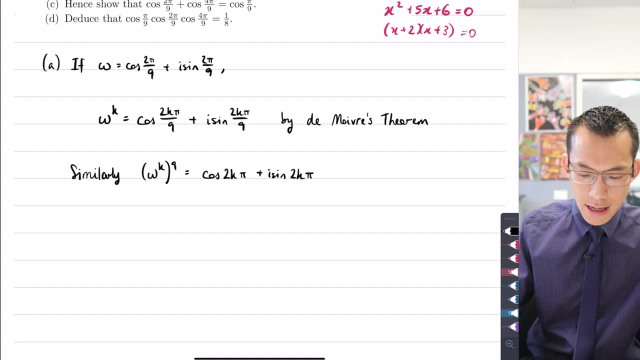 the integer power I raised by, in this case, nine. So what I get is, very simply, cos two k pi plus i sine two k pi. And what's great about this is that I now see I've got these trigonometric functions here which are periodic: every two pi radians. So cos of two k pi, if you have a think about. 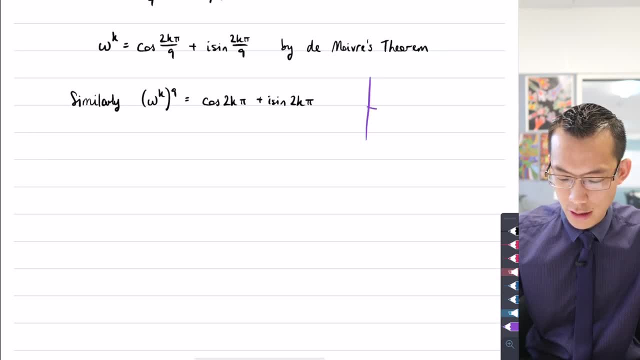 what cos is doing. let's just draw a really quick and dirty sketch over here. This is what cos looks like, right, So you can see. at zero, at two pi, it would happen. at zero, at two pi, it would happen. 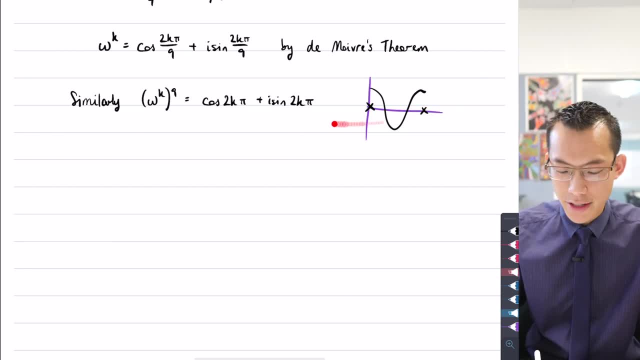 at. you know, if I kept on going to four pi and six pi, In other words, at every integer, multiple of two pi cos is equal to one. You can see it up there, right? That's the amplitude that you can. 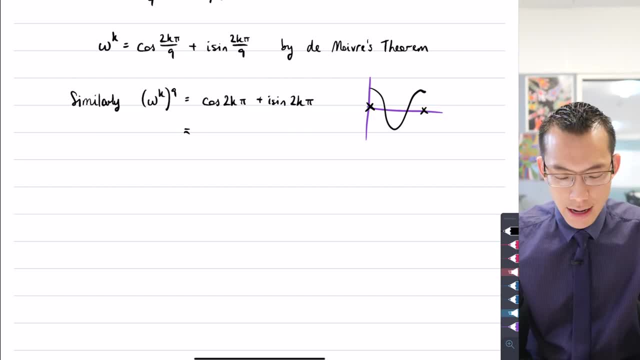 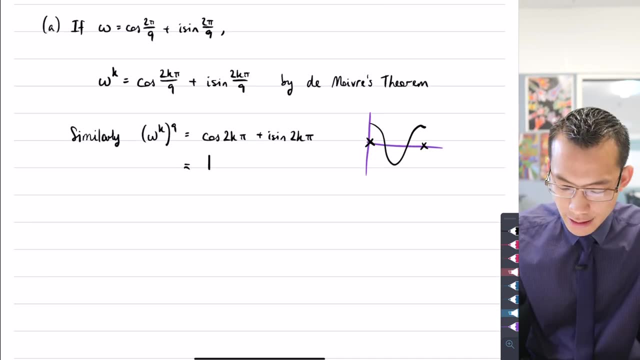 see there. So I've got this two k pi, no matter what value of k is, because I know k is an integer, I can say that's one. And similarly, if I get rid of this cos graph and put in its place a sine, 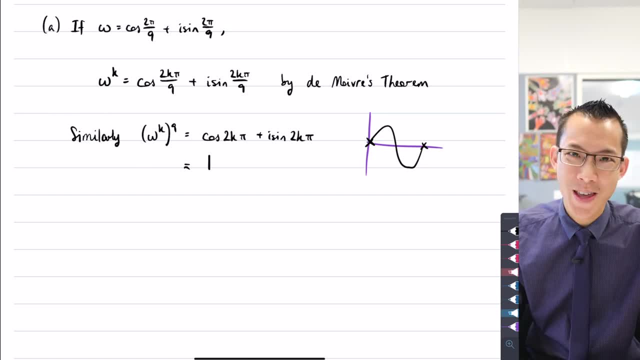 graph horribly messy, but I can still see the most important thing, which is that at all integer multiples of two pi like zero, like two pi like four pi sine is equal to zero. That's the value that it takes on, So I can say: plus i times zero. That's what happens to this And the reason for. 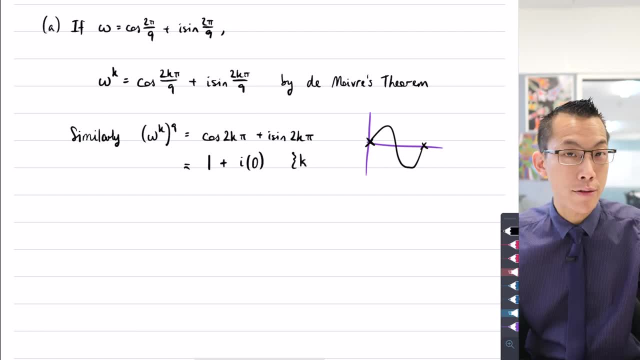 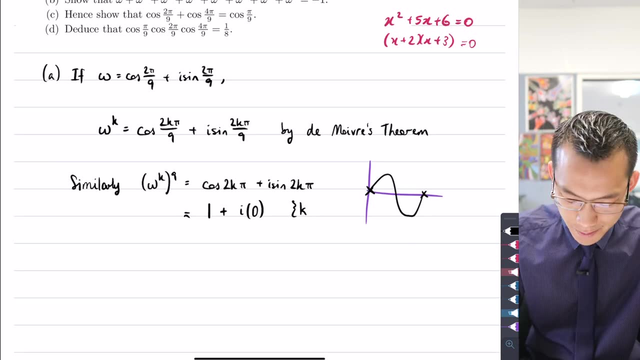 this is because of what I mentioned before, the fact that I have a domain restriction on k. k is an integer and that's the reason why you get these particular values. So, since that's my reason, I should quote it, I should invoke that fact. So k is an integer. That's the reason why I'm getting. 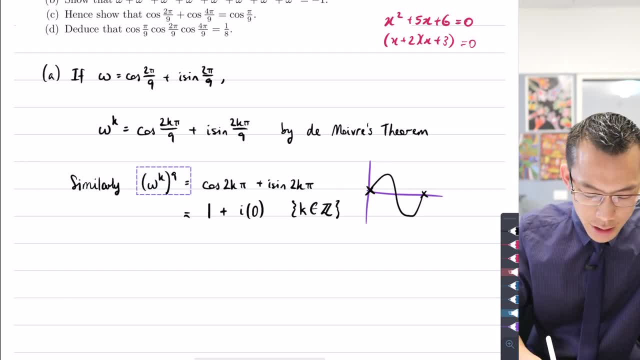 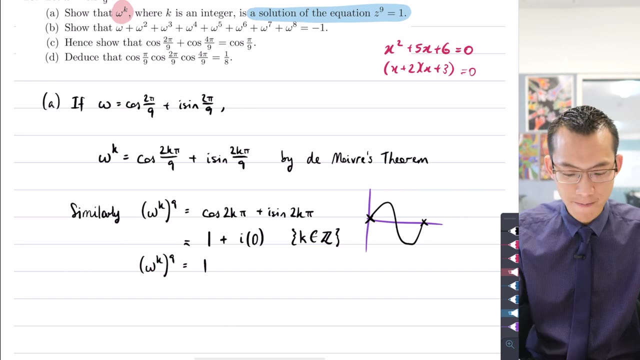 this simplification here. So what have I just shown? I've got this guy here equaling just. you know, this is zero, this is one. So because this satisfies, this is in the form: z to the power of nine equals one. it's just that this is my chosen z. that's enough to say this is a solution, right? 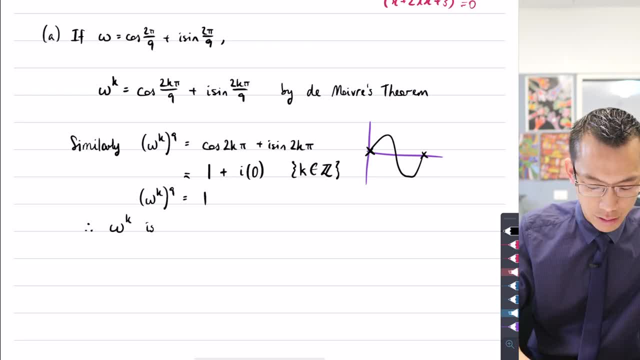 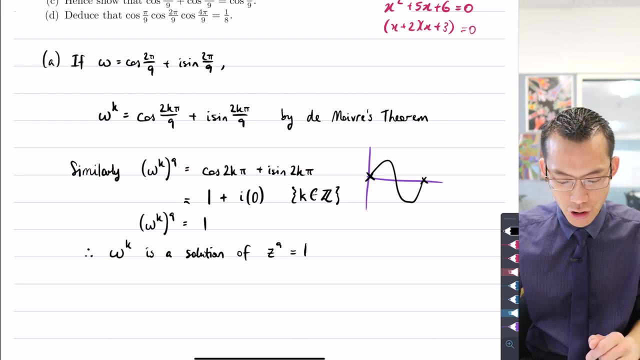 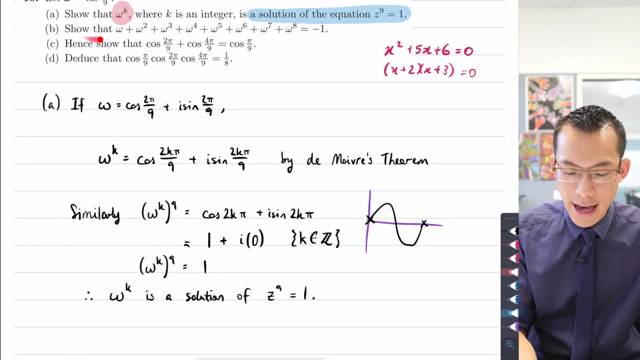 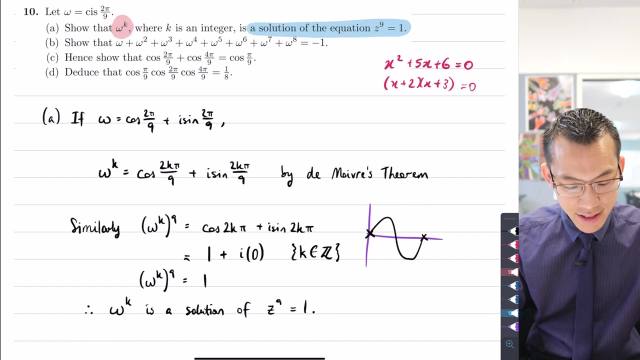 So I can say, therefore, omega to the power of k is a solution. That's all we needed. So that question is: how am I going to do this? Well, because this is a show question, right? I want to make sure my 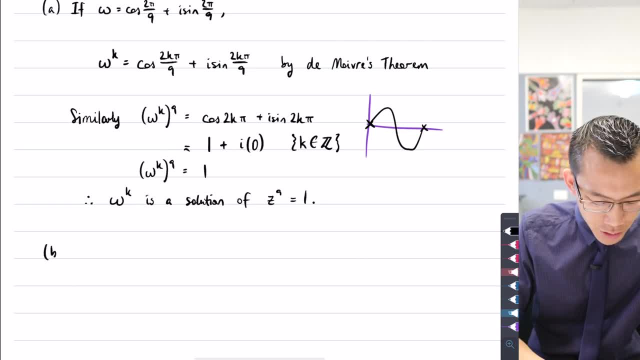 working is very clear. So what I'm going to do is I'm going to take advantage of a factorization that I know is going to be a solution. So I'm going to take advantage of a factorization that I know, but I I'm not just going to pull it out of nowhere. This is a show question. So I'm going to 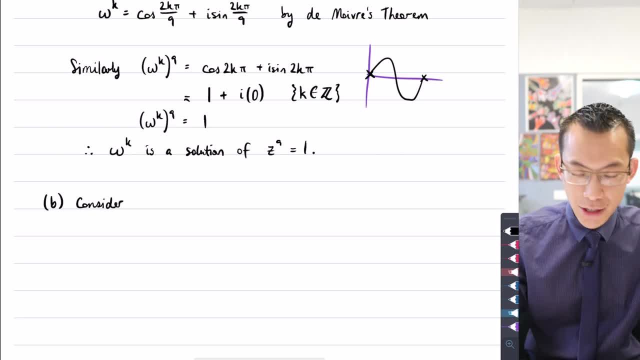 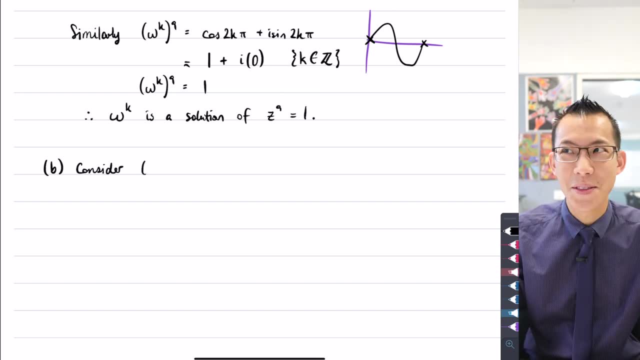 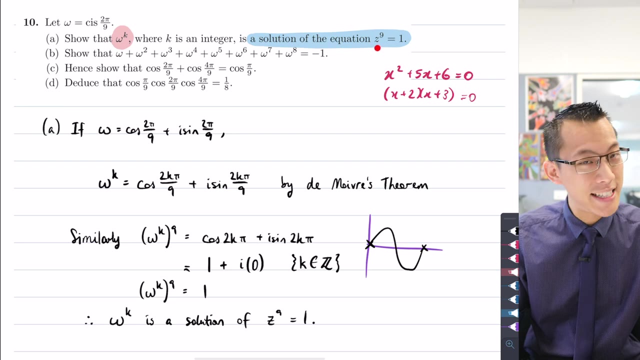 say: consider, because this is a result which isn't used like super frequently- it's going to be not the difference of squares, not the difference of cubes, but the difference of ninth powers. That's what I'm going to have here, If I consider taking this over to the left-hand. 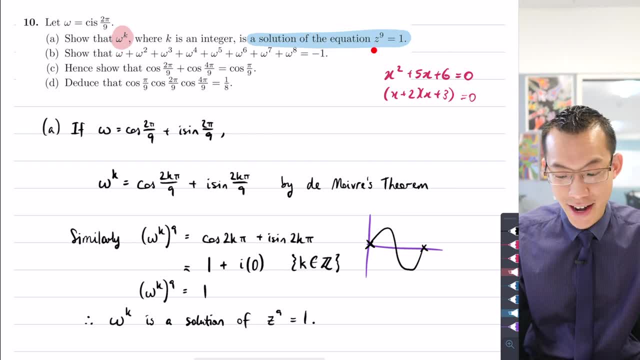 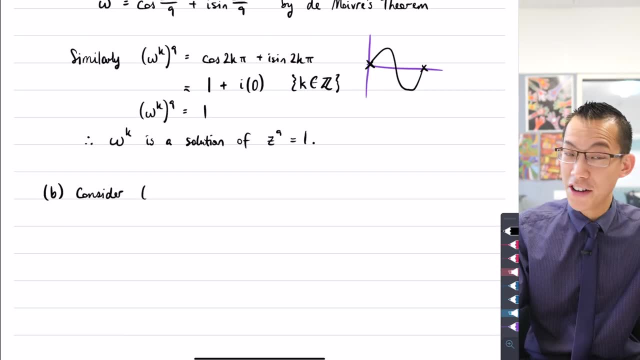 side, z to the power of nine minus one. z to the power of nine is the ninth power of z. One is also a ninth power. It's the ninth power of one. So, therefore, what I'm going to do is: I know in my 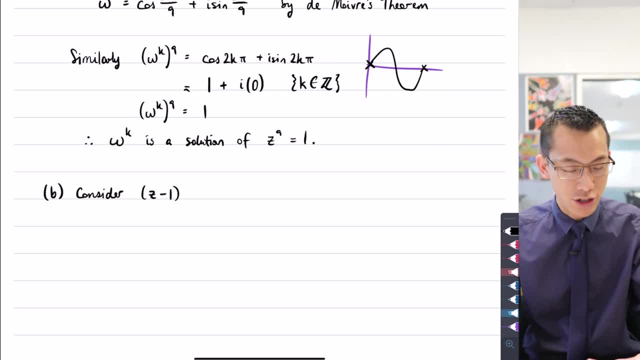 mind that actually this is going to be a factorization, but I'm going to have to prove that this is the fact, because the question does say show. So it's going to go like this And it's a general form. You may recognize this from doing you know the difference of squares and difference. 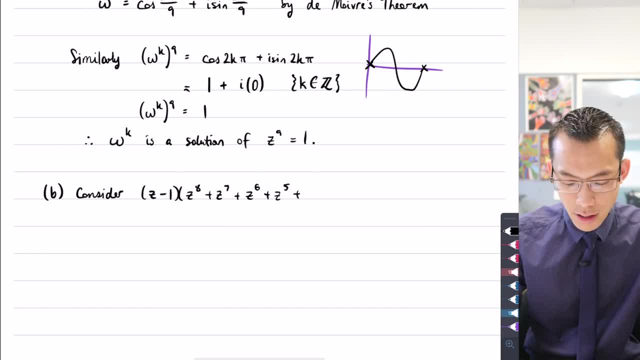 of cubes is just the smaller versions of this. So this goes all the way down, because they chose for us a very high power, All of this plus one. I'm just going to consider this right And I want to see what happens when I expand it. So I'm 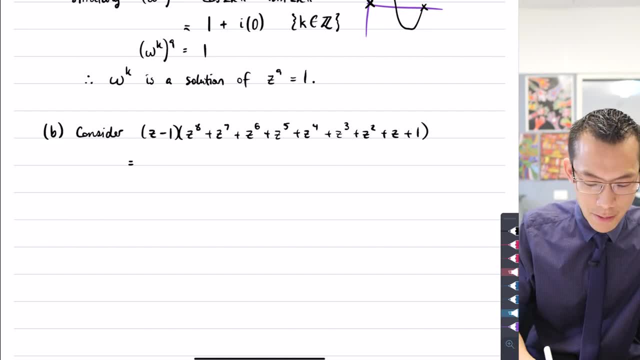 going to say: this equals two. Now what happens is, when I multiply z by everything here, this is going to become z to the nine, z to the eight, z to the seven, and so on. My last term will be a z. 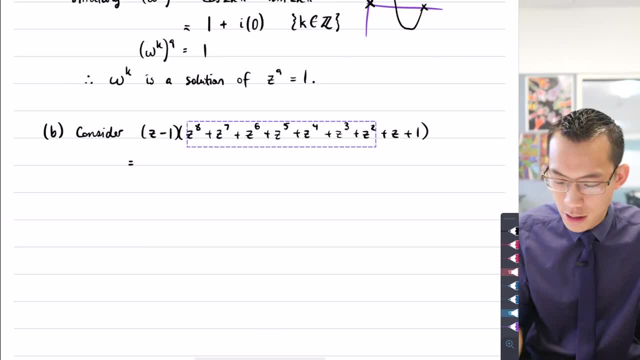 right. So everything ratchets up by one power. So I'm just going to be a bit cheeky and I'm just going to write all of those terms and then there'll be a z to the nine hanging out the front. So this: 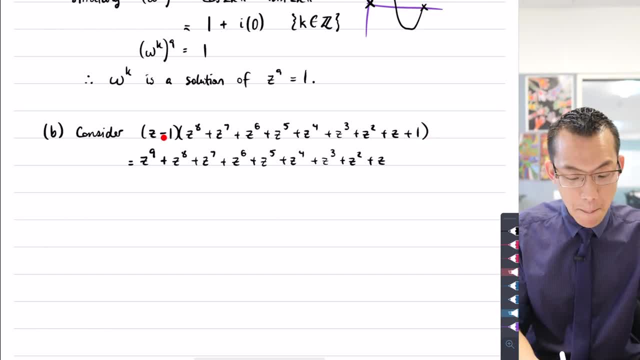 is just me expanding everything. What happens when I multiply everything by minus one? Well, you get all these same terms, but the coefficient will be negative one. So again, I'm going to be a little bit sneaky and take all these terms And then, instead of adding them, what's happening is I am 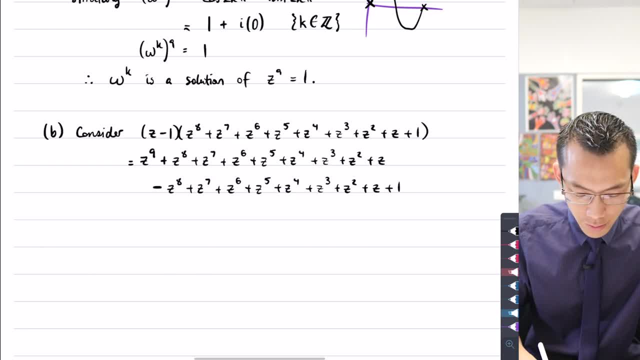 subtracting. That's the difference that this makes. So all of these become subtracted as well, Like I said. sorry that's a bit cheeky, but at least you don't have to wait for me to write all these terms out again. So this is just me expanding the whole thing in a very, very long 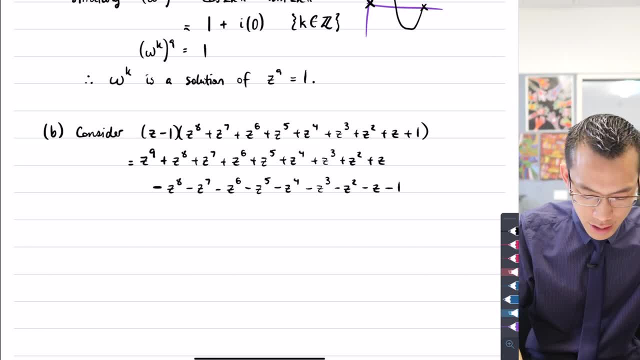 form. But you can see it doesn't take much effort to sort of notice that many, many terms are going to cancel in here. right, Your z to the sevens, your z to the eights, everything except for, you know, the z to the nine hanging out the front. no like terms for it to collect This. 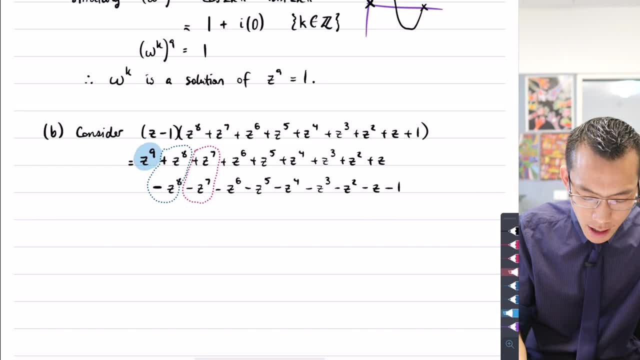 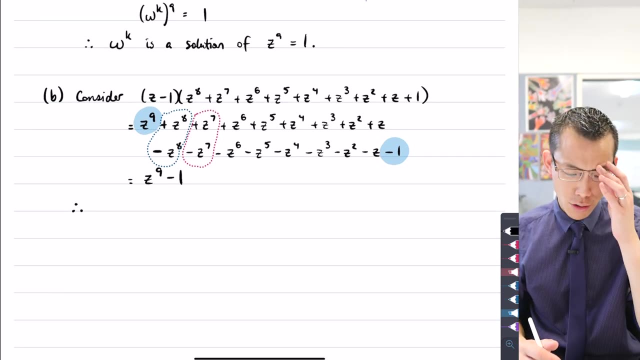 minus one hanging out the end. So these guys here will be your only remaining terms. So they equal to everything, z to the nine minus one. So therefore, I can say therefore, and remember, like if I weren't asked to show that this was a result, I would probably just go. 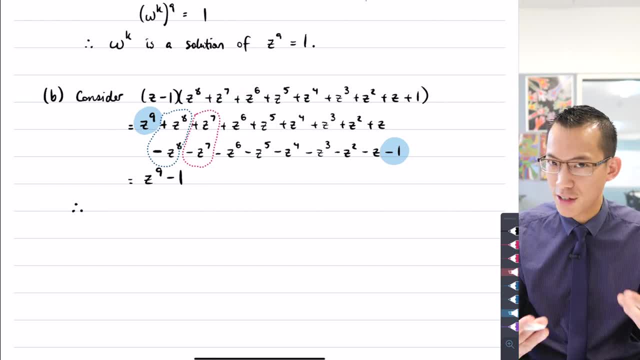 straight to this factorization that I saw on the top line, but I've been asked to show it, So I don't want just to come out of thin air. I can say, therefore, since oopsie daisy, let's actually. 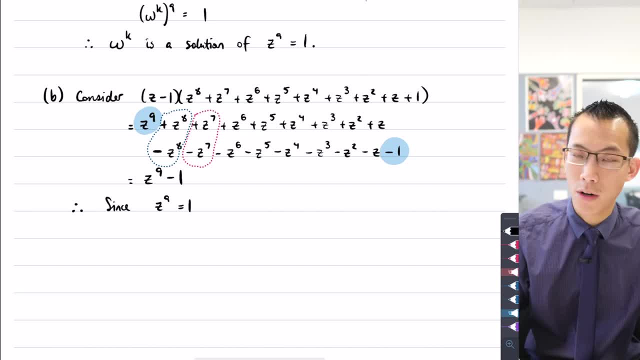 write this, Since z to the nine equals one. that's what I got from part A. I can say z to the nine minus one, that equals zero. but I just found an alternative way to write z to the nine minus one. I just showed the z to the nine minus one. 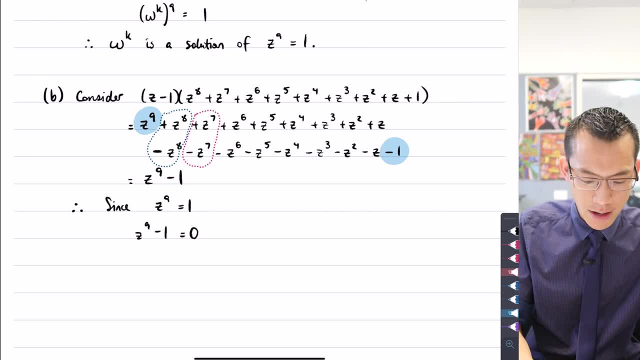 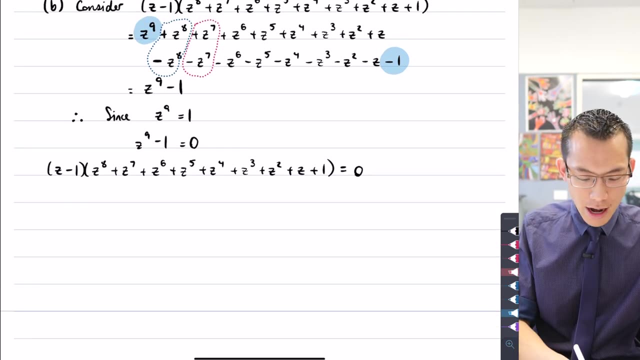 is equal to this factorization here, right? So I'm going to substitute this for my z to the nine minus one, So that equals zero. This is my new left-hand side. So how do I go from this to the result I'm after? Well, I can say: you know, I'm going to get a solution for this from z equals one.